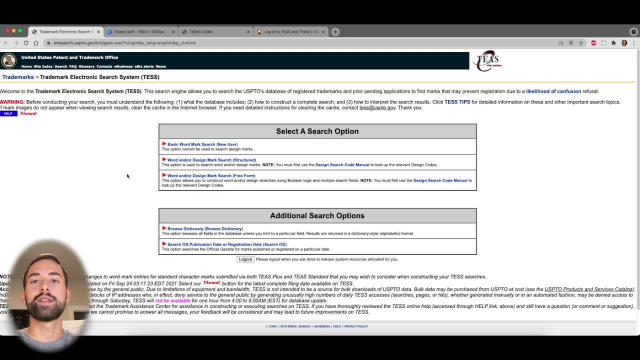 into the application for a golf brand that I'm trademarking and we'll finish it up. so you know what to do next. Okay, so the first thing that you have to do before you even get into your trademark application is to understand what it is that you're going to be trademarking. So 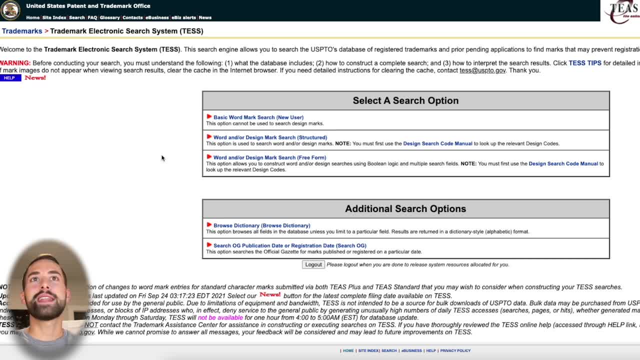 what your brand is and what are you trademarking For us? today, we are going to be trademarking the brand of Vibre Golf. It's Italian for to live golf. It's a brand I'm going to be using for some training aids coming up here in Q4 during the holiday season. So there's a link in the. 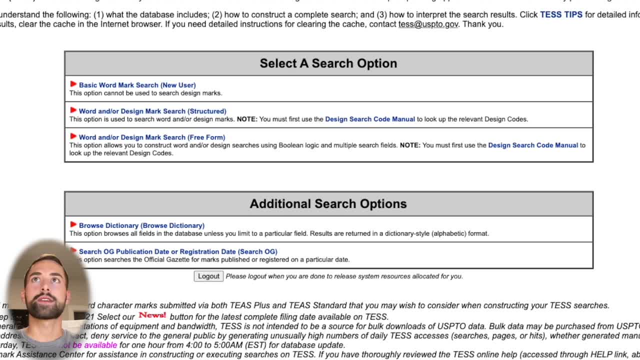 description and this is going to be our trademark. sorry, trademark electronic search system. We're going to search for that trademark brand and you're going to be searching on your behalf for your trademark brand to see if someone is actively using it. If someone is actively using. 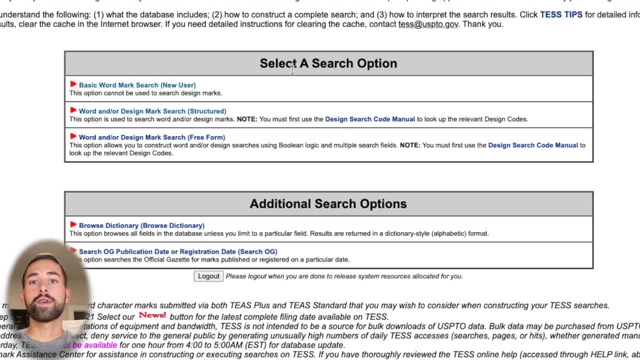 your trademark. you cannot use that, So you're going to be searching for that trademark brand, so you'll have to find a new brand name. So the first thing that we're going to do is we're going to go to this section where it says select a search option, and we're going to click this first one. 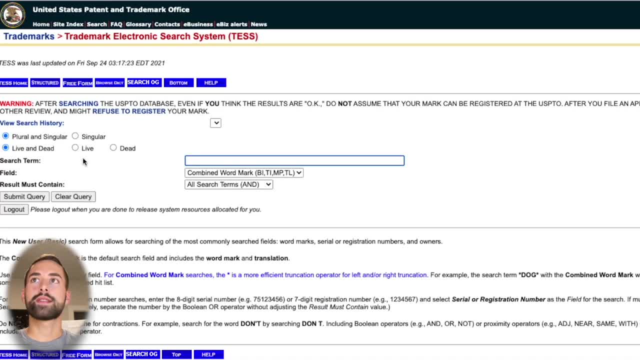 where it says new user. Once you click that, there's one thing you have to do on the left here, and then we're going to type in our trademark brand. I usually filter this down to just the live trademarks. I really don't care about the dead trademarks that aren't active- and then I'll 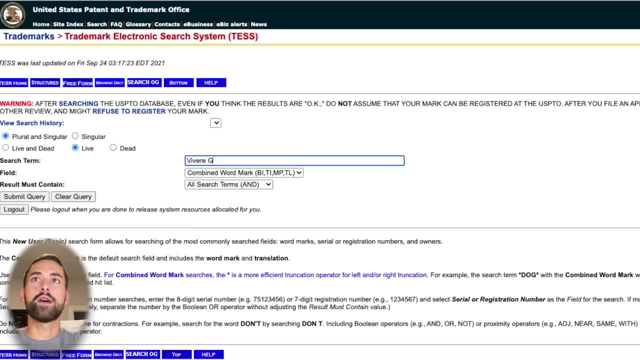 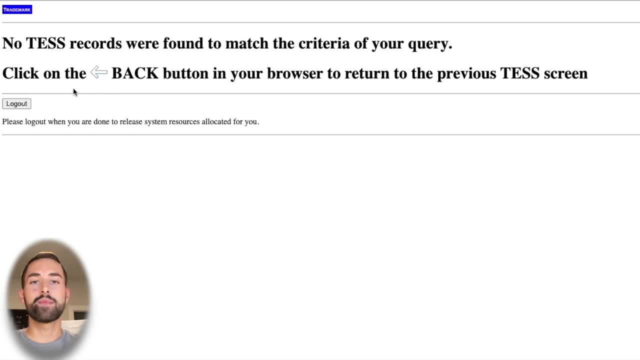 go down to search term here. So again, ours was Vibre Golf, with a space between them. Type in your trademark here. After you do that, click submit query And you're either going to be brought to a screen where it says there are no records found. 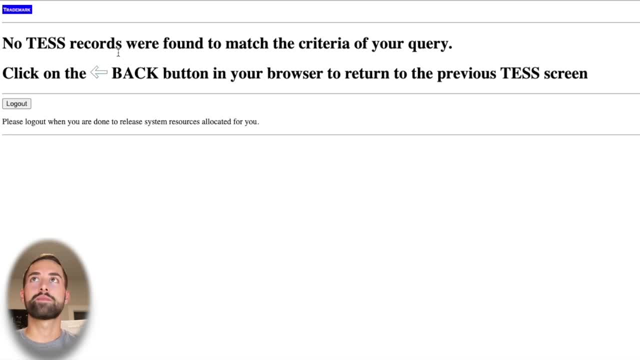 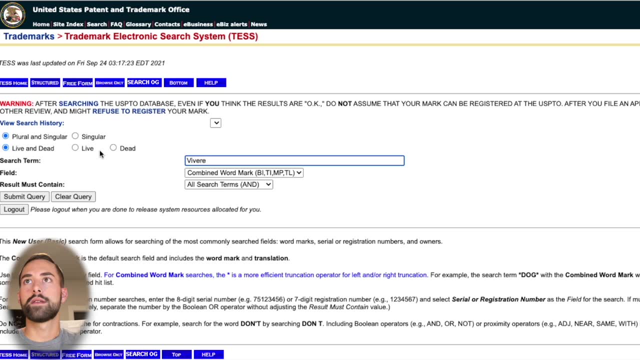 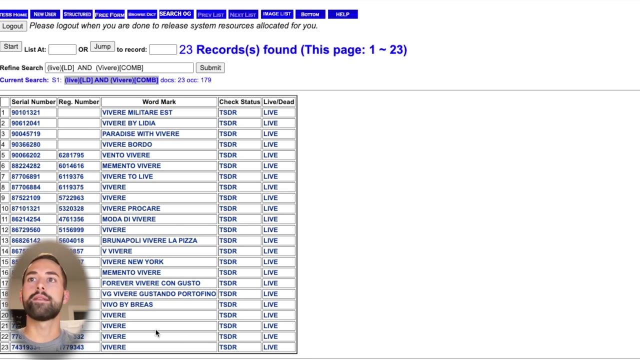 which is great. That means that I can use and trademark this brand name as is. Now. let's go through an example where we do find- So I'll just type in Vibre live trademarks And, as you can see, there are a lot of live trademarks just with the Vibre name in them or by itself. So if you come, 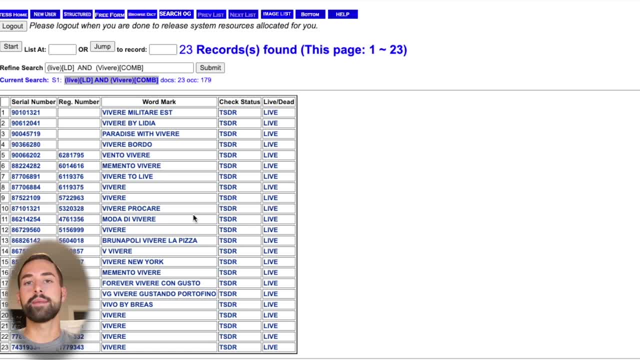 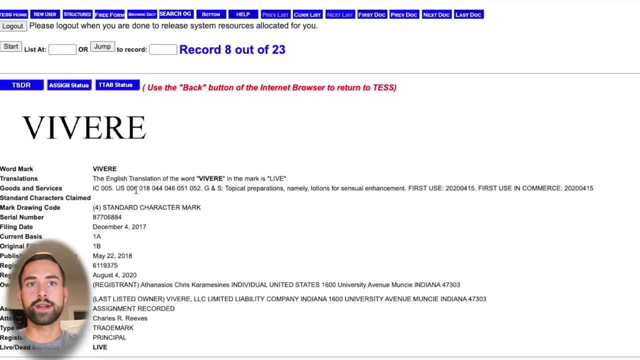 across here and you see a lot of trademarks that have the existing brand name that you want to use. odds are that you cannot use that. I mean, you could go into each one of these and see what class they are trademarked under, but it's really going to take a lawyer to come in here and fully understand if you can or cannot do. 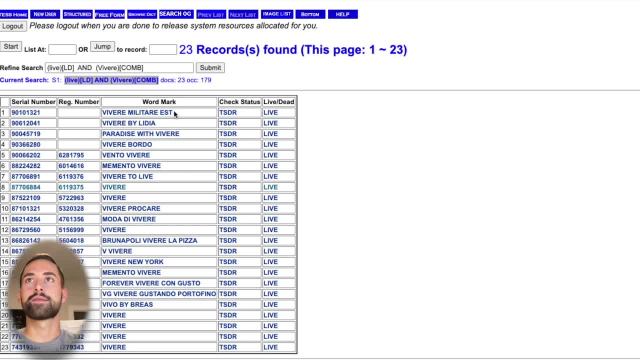 it. My word of advice is: if you have all of these listed here for your trademark name that you want to use, go ahead, find something different. It isn't the end of the world, So for us, when we searched it for Vibre Golf, it was not located on here, So that's assurance that I can go ahead. 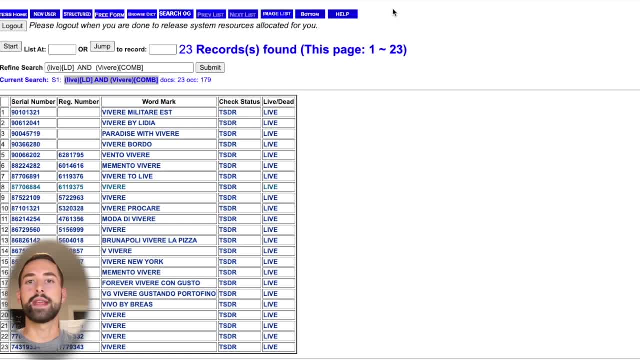 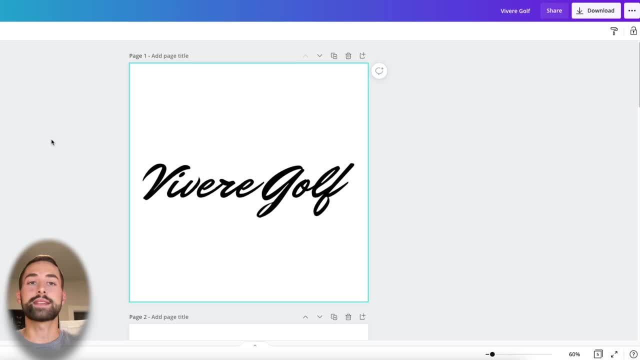 and proceed with my application and I can make sure that it gets submitted and approved. Next we need to go and figure out if we're going to be doing a logo for our trademark or if we're just going to do basic text. So I want to do a logo that has this cursive like text- It's Dr Defoe text, So I'll be doing a. 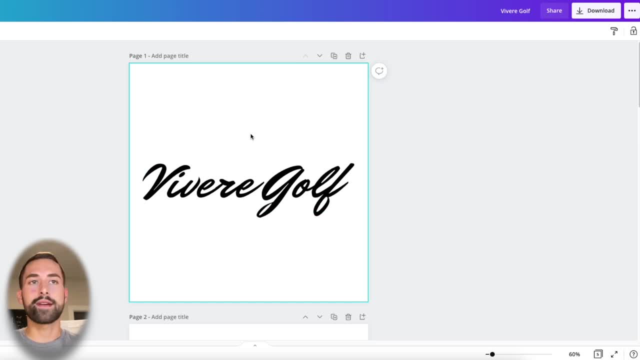 logo for this demonstration For you. if you really don't care, if it's the design of the trademark itself, you can just do a basic formatted text and you don't have to go through this entire process. However, if you do want to do a logo, make sure you use some type of software to create. 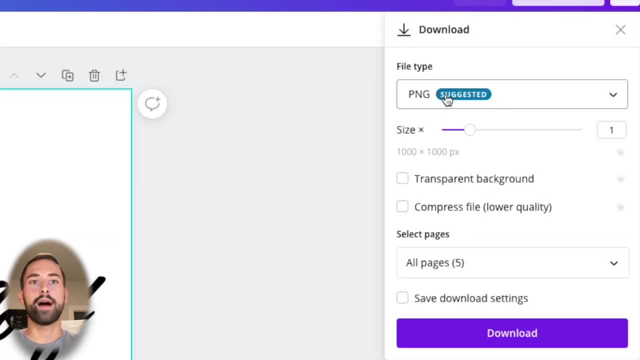 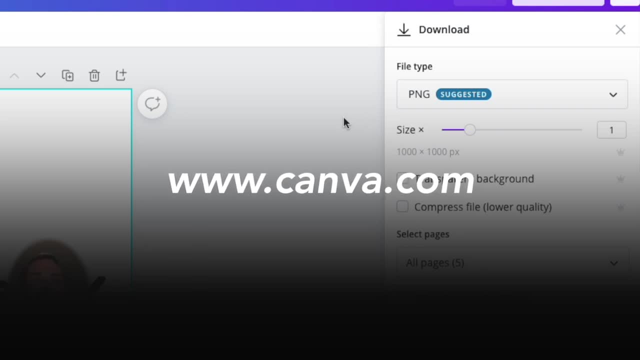 it like this, And then you're going to want to save it as a JPEG file. I'm using Canvacom, great free online software that you can use. You can go ahead and create free logos, such as this simple one right here. Make sure that you save it in a JPEG format. 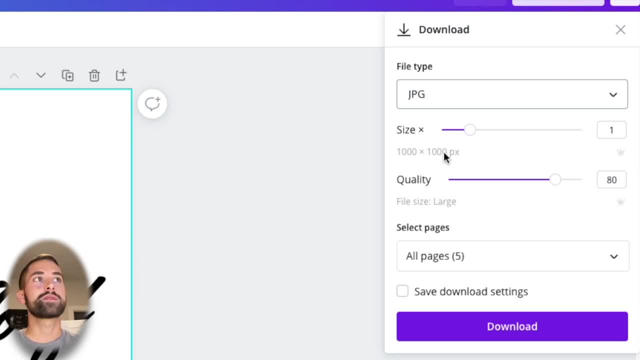 because that's the only format that they will accept. And then you want to make sure that your file size is under. I believe it's 944 pixels on either side. As you can see, this is a thousand by a thousand. It's too large, So we need to reduce that down to 500 by 500.. I think the minimum is 250. 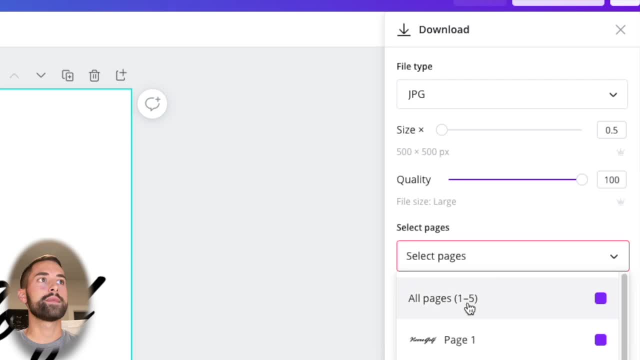 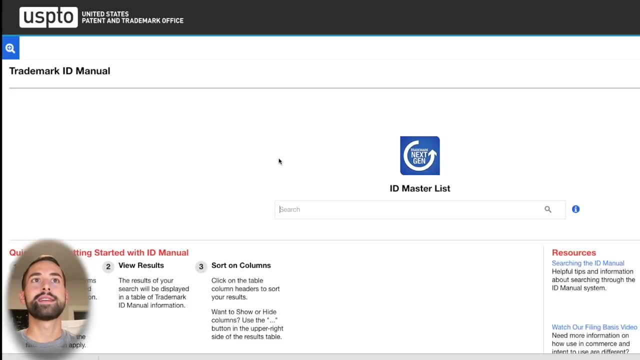 pixels. So just make sure you're within that and turn the quality up, and then I will save this and download it to my downloads folder. All right, so that's step two. We're almost there to the application. Step three and the final step before we can actually get into the application and 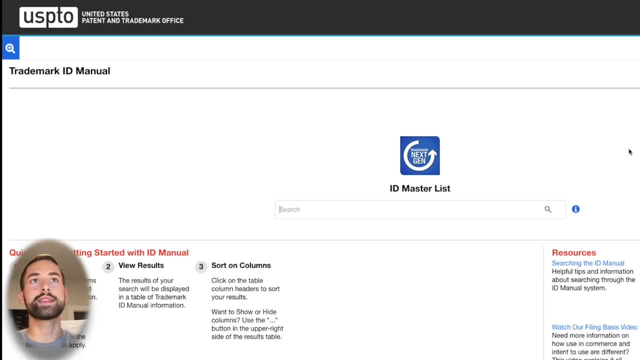 please do these steps because it's going to save you time. The last thing you want to do is submit an application and it gets denied by the government because you didn't follow some of these steps or you didn't do your due diligence that you need to. Next, we are going to be searching the trademark. 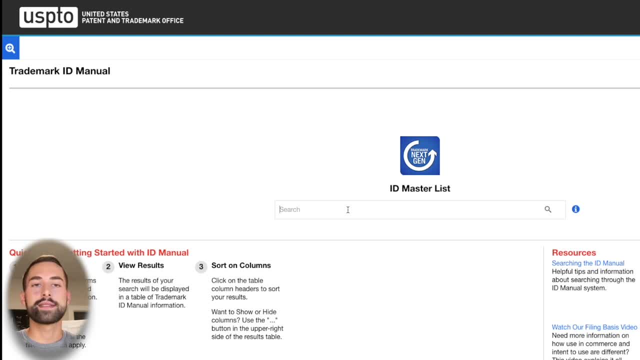 manual. So this manual is an assortment of all these classes that are filed and services on behalf of people like us and companies. Now we need to search this because, in order to decide if we are going to go with the TEAS Plus or the TEAS Standard application- two different applications. 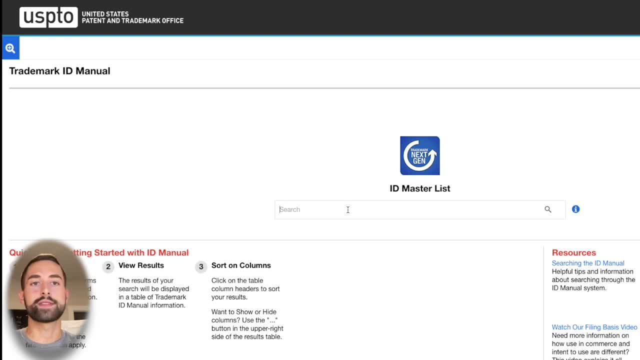 we need to make sure that there is a class that's out there that relates to our product. If there isn't a class that relates to our product, we're going to go with the more expensive option, which is the TEAS Standard, and it's about $350 per class. 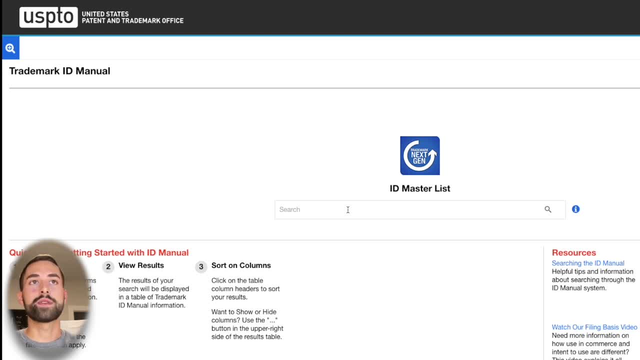 So let's say that you have a brand where you are selling wallets. You go ahead, you fill out this application. you get your trademark for that specific class. Now that does not mean that you can go and use your brand name to sell stereo equipment or lights, because that trademark is. 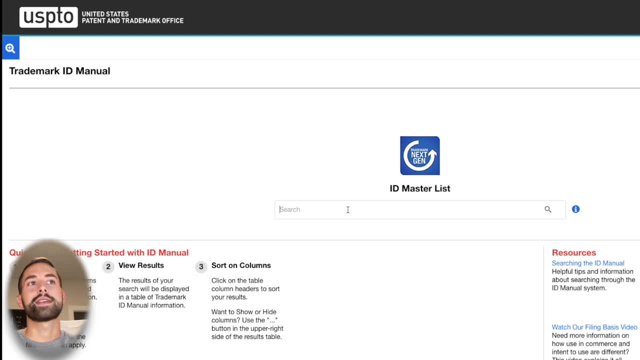 only eligible in that class or service. So that's one thing to keep in mind- is that you're only trademarking within a specific, narrow niche per se, and that's one thing you have to keep in mind when you're going about this. So, in here, what you want to type in is what your product is So for. 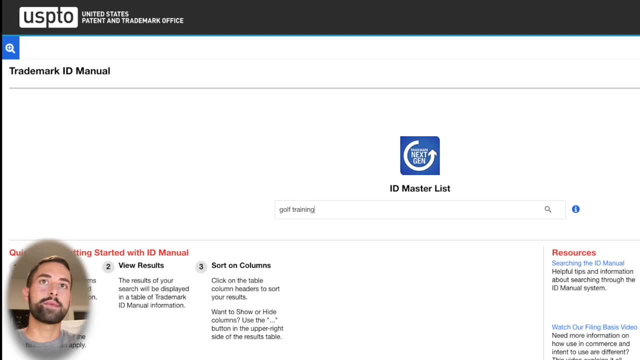 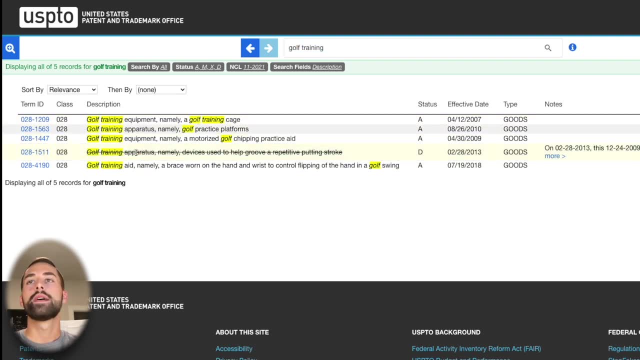 us. it's going to be a golf training aid. I'm just going to type golf training to see what we have. So you can see a bunch of different classes come up. Do not pay attention to the ones that are strikethroughed And then just focus on the ones that relate to your product. So we're going through. 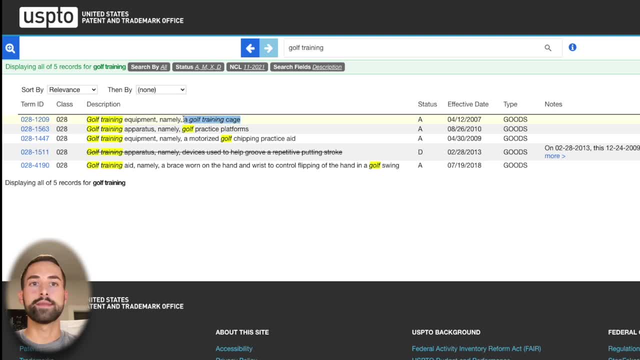 these. It's a golf training cage that would not relate to my putting device that I'm creating. The next one, golf practice platforms. It's a golf apparatus that would work for what I'm doing, And but I'm going to take a look at the rest of them just to make sure. 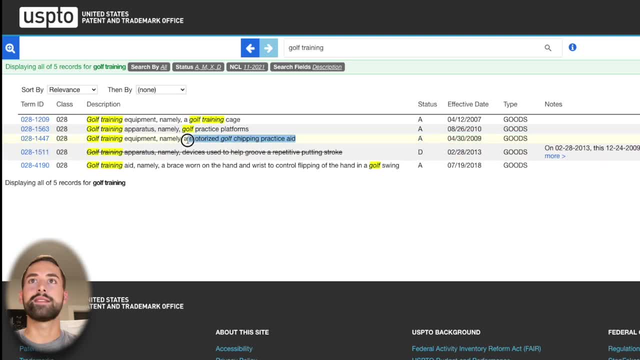 This third one down here: a motorized golf tripping practice aid. Nope, mine is not motorized and it's not a brace that will be worn on the hand. So if you type this in and you can try a couple of different searches, maybe golf aid next, But if you find one, that's good news. 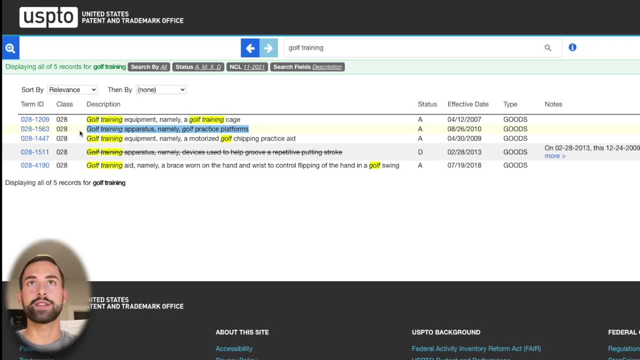 You don't have to really remember this yet, because you will search this later on the application. But if you search this and you couldn't find anything or anything that related to your product, you're going to have to go through the TEAS standard application. All right, So at this. 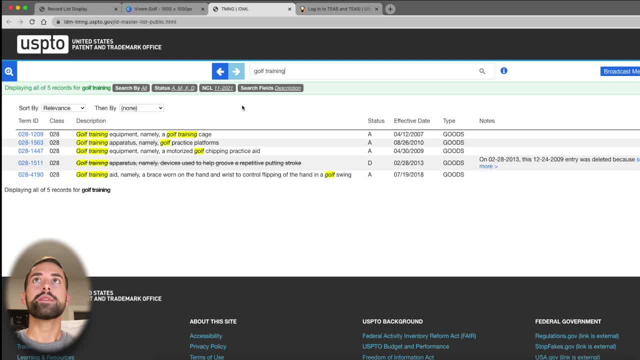 point. we've completed all the due diligence steps, So we're going to go ahead and type this in. We've done all the steps that we need to We ensure that our trademark is not actively listed. We created our logo if we wanted to, And then, lastly, we found a class and a description that 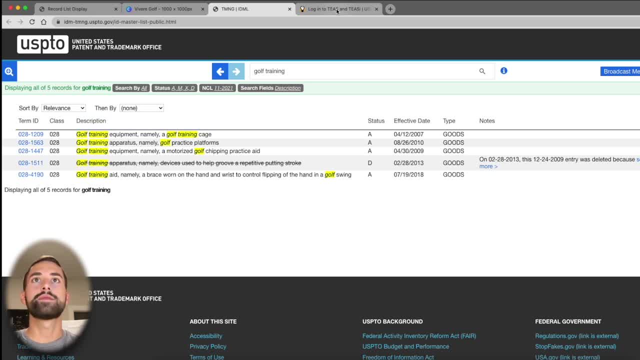 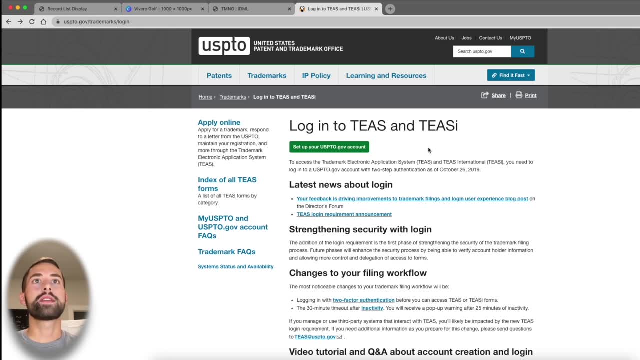 fits what we're trying to brand here. Next, go down to the links in the description and go to the actual application link. So now we're going to actually get started with the TEAS and TEAS I application. First, you need to go to this green button here where it says: set up your USPTOgov. 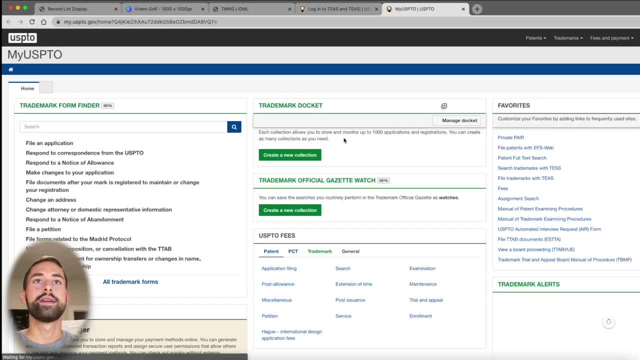 account. if you don't already have one should already be logged in Now, after you've actually created your account. it's very simple: just type in personal information and then, once you create your account, you'll have to verify your email address and then you'll be brought to this dashboard. It's very easy what to do next? all you. 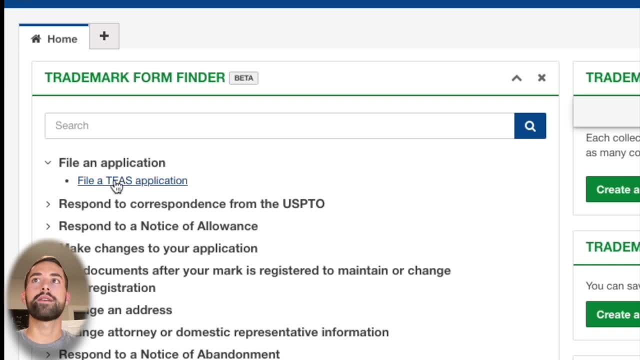 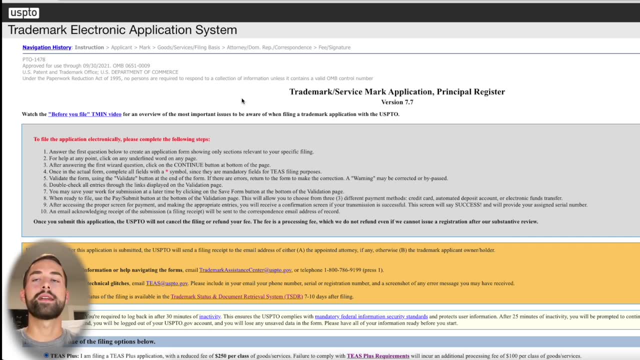 have to do is go to this file an application and click file a tease application. Now this is the actual application and we're going to go step by step through it with that golf brand that I'm looking to trademark. Now you don't have to read all this text, because you're just going to follow. 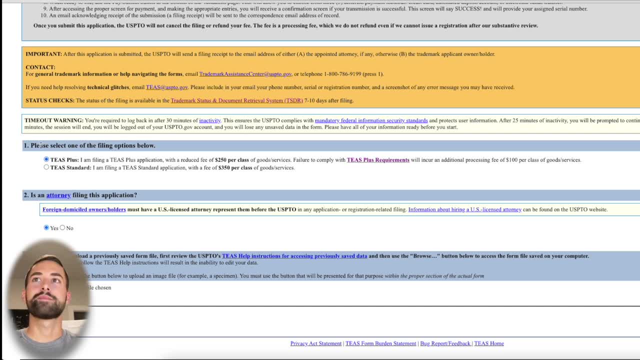 the video and I've already done it for you. So the first question is: please select one of the filing options. You've heard me say tease plus and tease standard. remember, if you're doing a tease plus, that means you were able to find a class and description that fits what you're trying to. 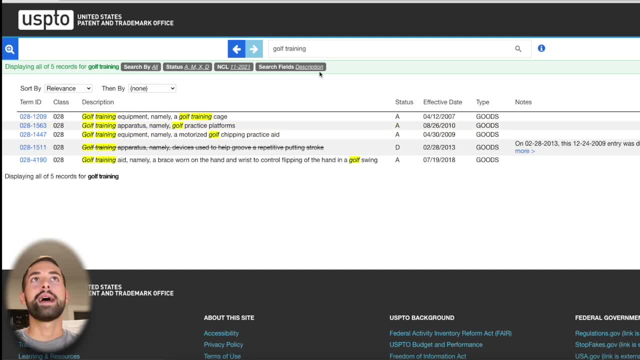 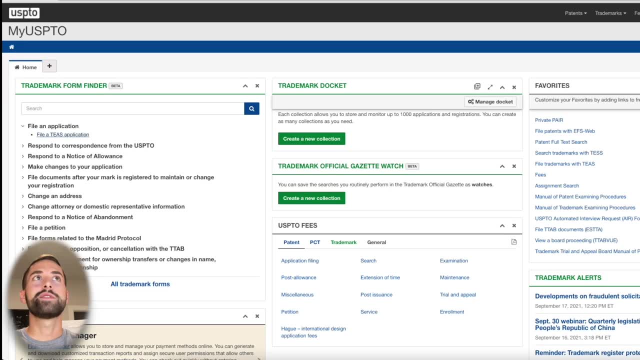 brand and what you're trying to sell For us. that's what we'll do. however, you're going to do tease standard if you couldn't find something that relates to your actual trademark and do not try to bend the rules here. a lawyer is going to look over your application. 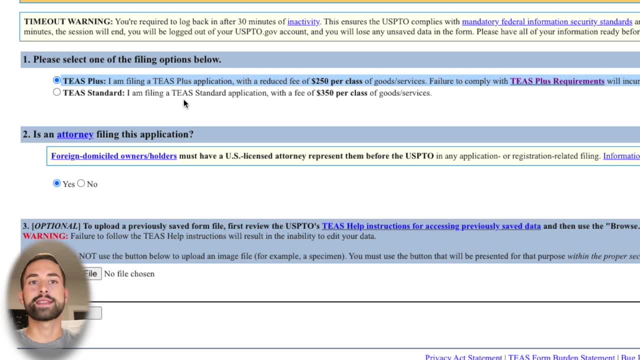 and they see that there isn't an actual class and goods that's already existing in the id manual, they're going to reject your application and tell you to file t standard anyways. so it's not an opportunity to save money, it's really just the luck of the draw for you, okay, and the second. 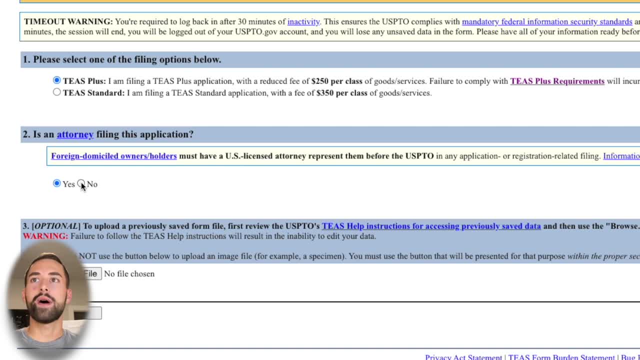 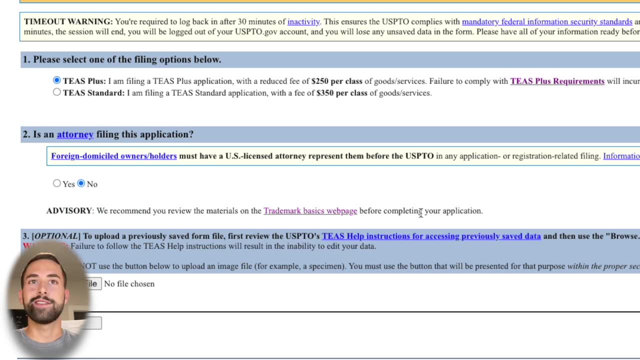 question: is an attorney filing this application? no, i am not an attorney, and you're going to notice here. saying we recommend you review these basics before completing your application does not say that you can't do this because you're not an attorney. save some money and you can do this. 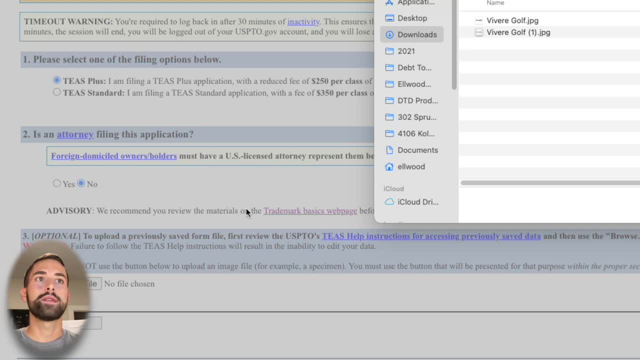 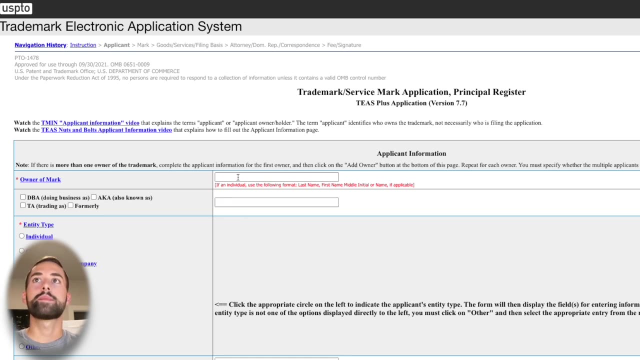 by yourself. this is an optional third one here, when you don't have to actually go ahead and complete this next click continue and this is where you're going to describe your ownership and who the applicant is. now, i am just the single person that is filing this application. 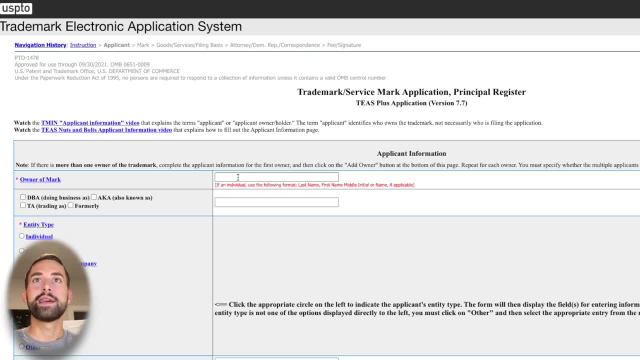 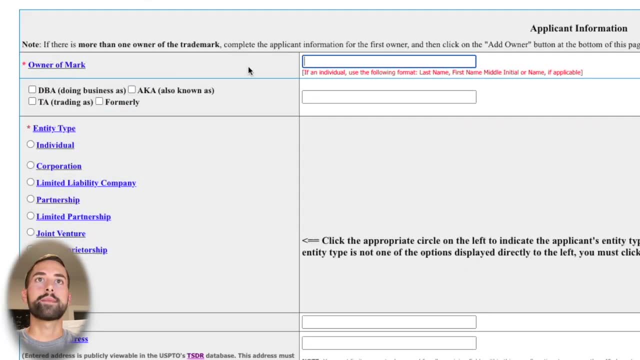 say, you have a partnership with a couple different members for your business. you want to include everyone on here. that needs to be, and you're going to be able to do that. at the bottom you can add multiple owners. so for the owner of the mark, i'm going to type in my name here, so i'll say: do in. 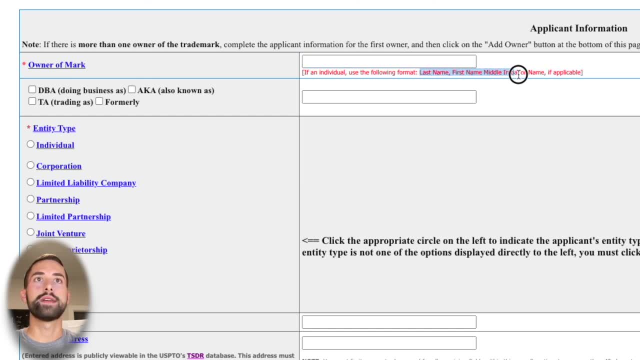 the format of last name comma, first name, middle initial. so i'm going to type my name in. if you're doing business, as in another business such as llc, as i will be, i will type in that business here and then, down to the left here i'm going to select the entity type for my business. 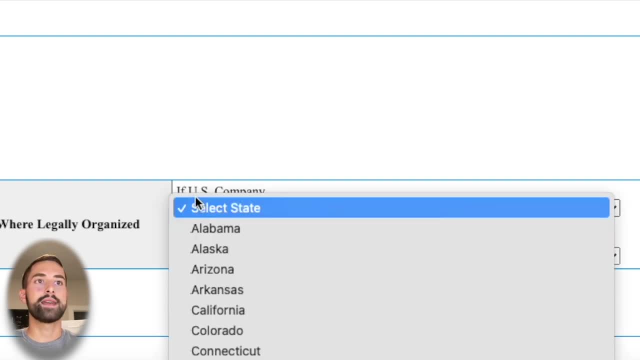 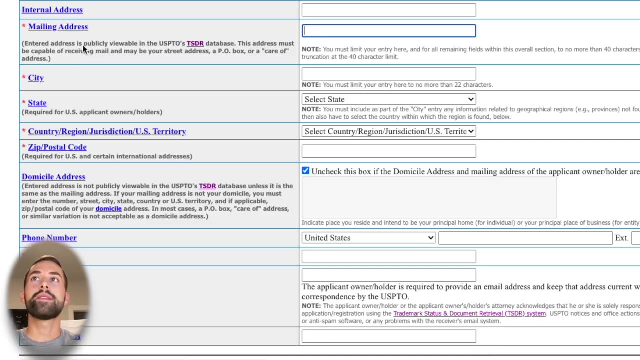 for me it's a limited liability company and you need to select the state that your business is legally filed under. okay, next we'll skip down here to your mailing address. keep in mind this is going to be public. it's going to be viewable by anyone looking. 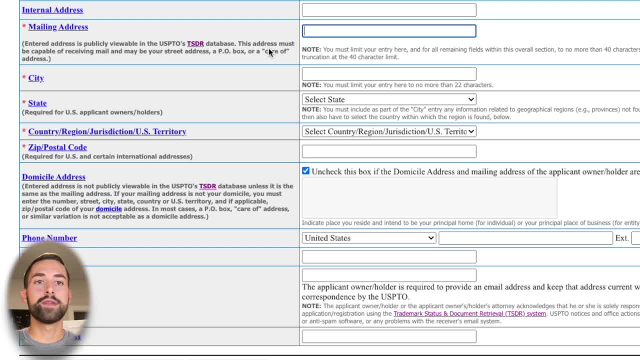 through this database. so if you do not want your address being publicly viewed, i would go ahead and get a po box just to protect that, so you're not receiving spam mail or having anyone creepy show up your house. so type in your address here, okay, and then we'll leave this checked phone number. 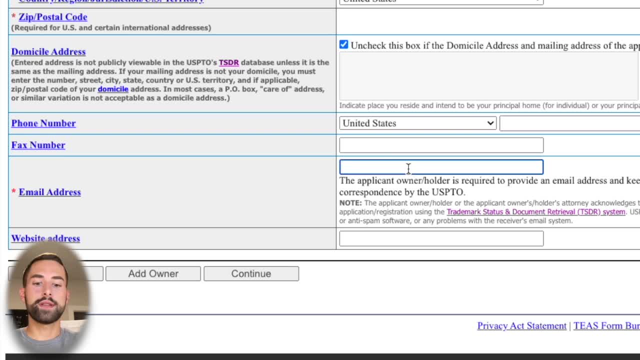 you don't have to put anything in here- fax number you don't either- and then just put in your email address. all right, so at this point, once you have all your required information in here, you can go ahead and click continue. if you do have more than one owner, click add owner and then you're going to 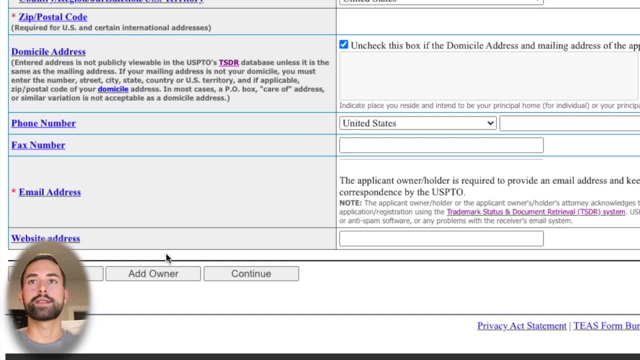 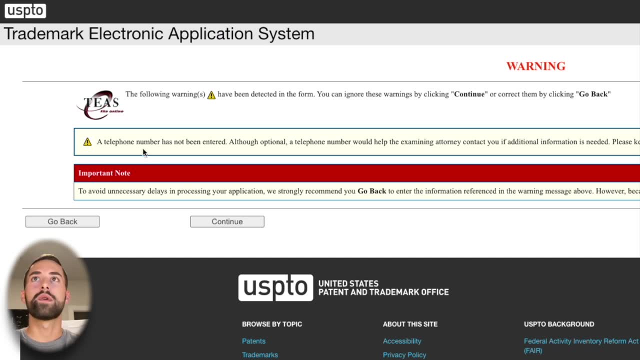 see the owner and that will add this first person, and then you can add the second, third and so forth. once you've added all of the owners, click continue. now, since we did not put in a telephone number, you're going to get a warning message. it's only a warning, it's not a requirement. so if you want, 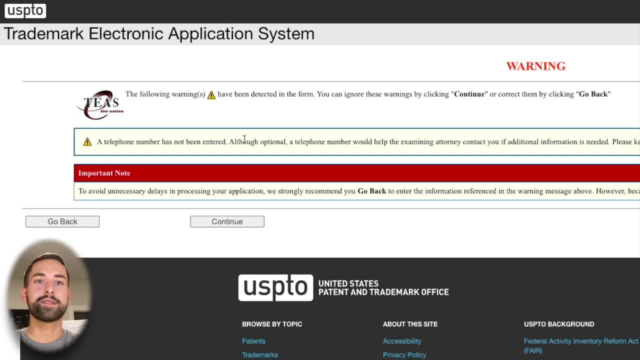 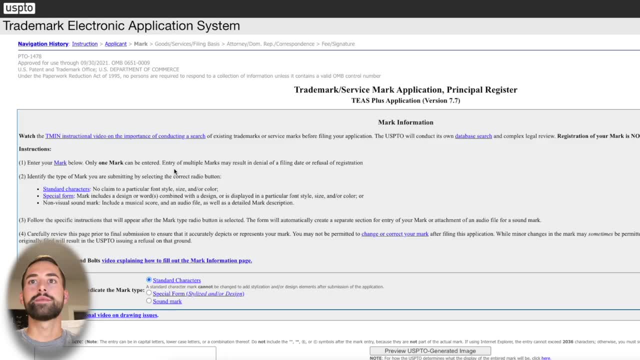 to go back and add your telephone number so an examining attorney or someone can contact you. you can do so. i'm just going to click continue. i don't like to have my number out there, just for the sake of that. okay, and the next step is our actual trademark. 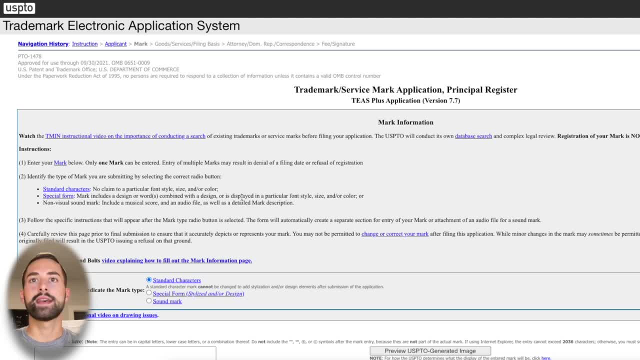 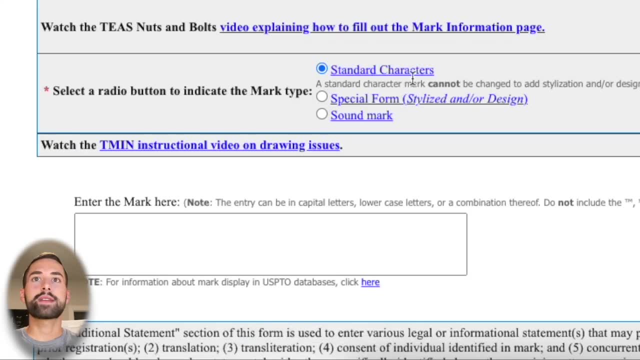 upload our logo or we're just going to type in our standard character text if you do not have a logo. so the question you're going to answer down here is to select a radio button to indicate a mark type, standard characters. again, that's just like plain text. so this would be. 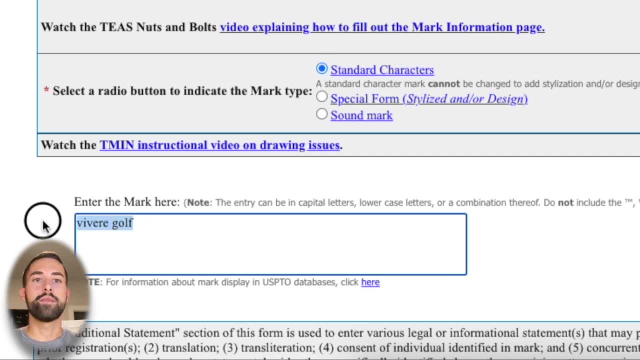 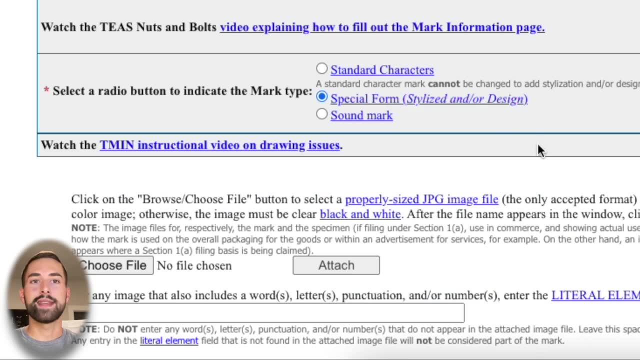 my trademark. if i were to do plain text, that's all it would be right. there's no design to it. i'm going to do a special form which is stylized or design, or better known as a logo. so now we're going to actually upload our trademark, our logo, that we saved beforehand- again they say to save- 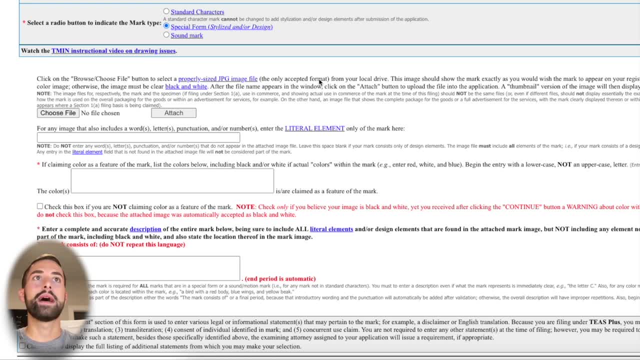 it in a jpeg image file. it's the only acceptable format. some other things: if you're going to trademark colors, make sure you upload the color format. otherwise black and white is fine for us. we just had black text, so we really don't worry about the colors and all you do now is go to. 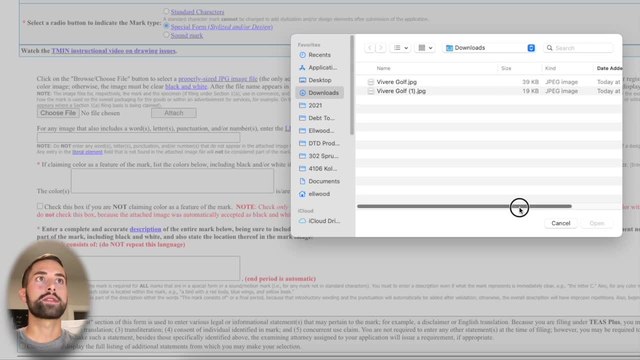 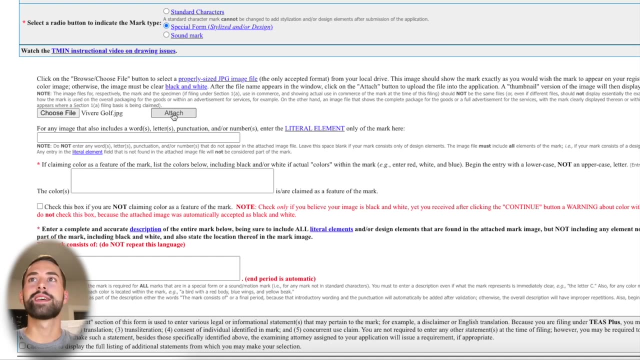 choose file and click the one. let me make sure i click the right one here. it says top one, so you click that and make sure you click attach, because that's something i did first. couple times i tried doing this. you get to the end and you never click attach. so this actually attaches it to your. 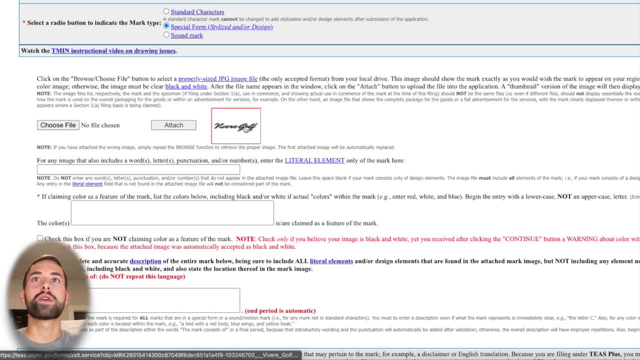 at that point you should see your trademark brand, your logo, right here. just ensure that it looks correct. it's going to be a little bit distorted because it's very small there, but that's that's it there. now. at this point, you need to type in your literal element, which is down below here. 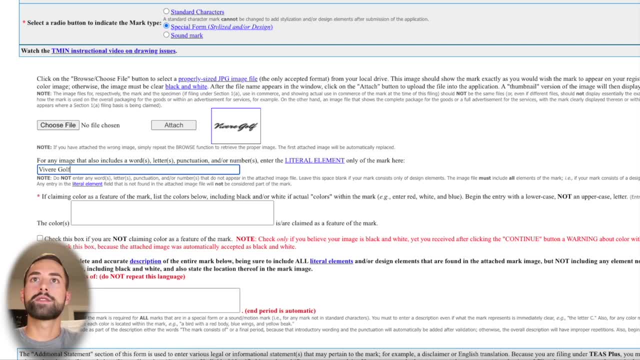 type in exactly what your trademark says. uh, you have to do this just in case you know the examining lawyer. they try to examine this and they couldn't tell if this was a w or a v, or if the g was you know something else, or there wasn't a space. so just type in the text, if there is text. 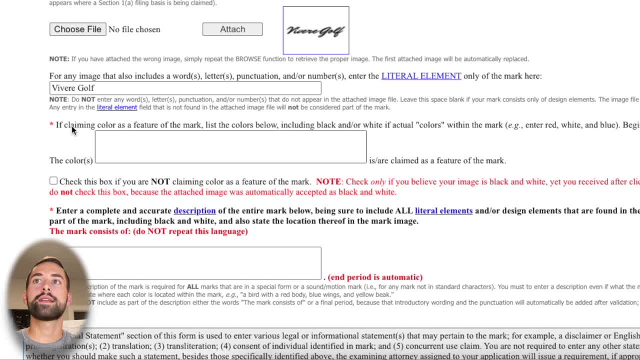 and then you're good to go and put that there. okay, and moving down here, if you're claiming any colors as a part of this logo, then you have to make sure you enter them here. this only applies if you have colors that are not black and white. so for us we're going down below here. it says: 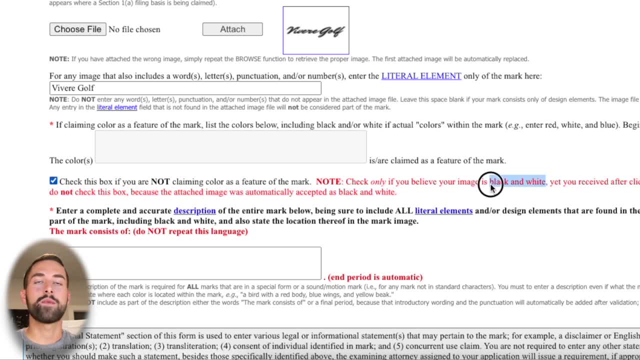 check this box if you're not claiming a color. this is really only for black and white images. now, what you would do here, say this, was a, a red v and a blue g. we want to indicate that here, so we put red and blue, so we'll make sure that both of those colors are actually a feature, a color feature of our. 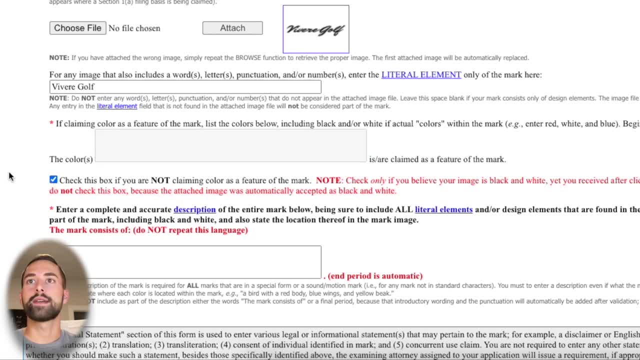 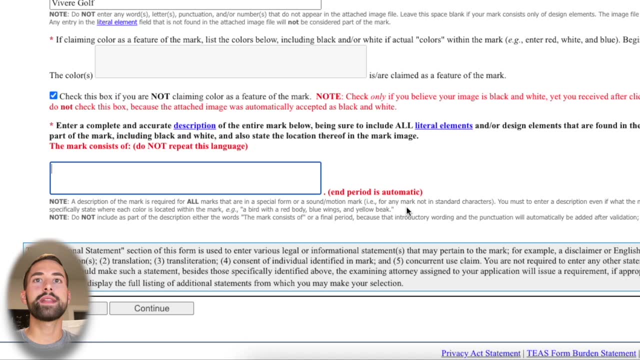 trademark, but since we're just doing black and white, we'll leave those out of there. next we have to add some more descriptive elements to our trademark to describe what is going on now. if you have something that's very complicated or an actual logo without text, you want to indicate all. 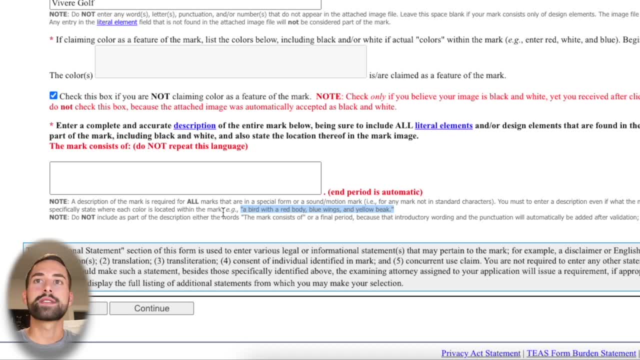 the different colors and the unique aspects of that logo. so for down here here's a good example. if we had some logo with a bird with different colors on it, we type in a bird with a red body and a yellow beak. that describes our trademark logo. make sure that you start this field without 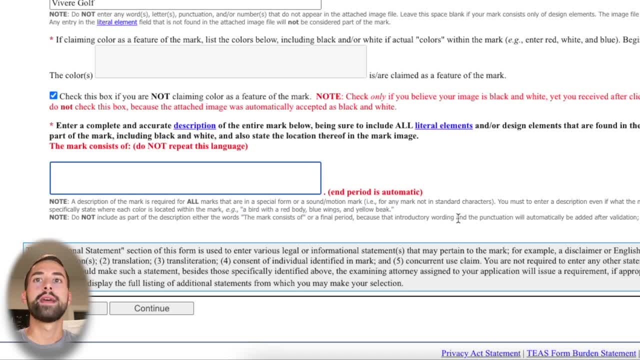 an uppercase letter. keep it all lowercase format and do not start out with like a full sentence, like you would. this mark consists of, or this trademark resembles this. just type in exactly what it is: fever, a golf, all black. let's just put color, okay, so that describes it there. after that: 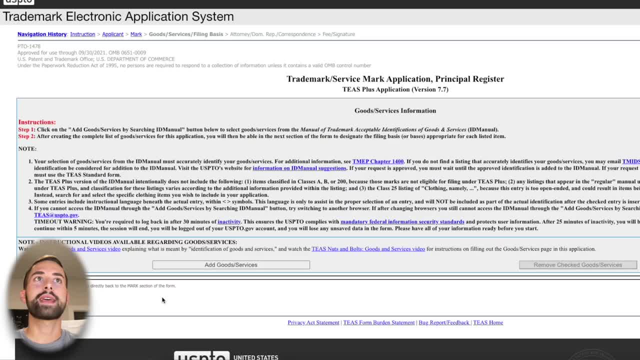 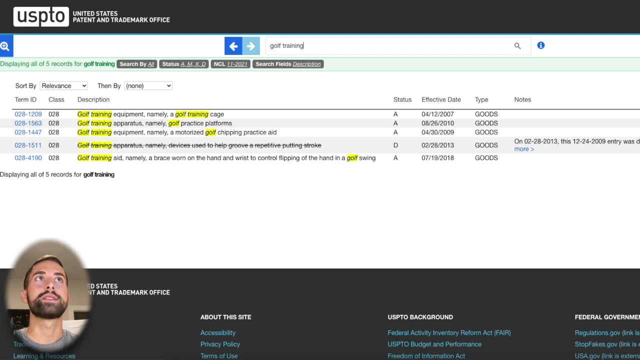 you can click continue and it will be. you'll be taken to the next screen, which is actually adding your trademark to a specific goods or services. now this is going to look very similar. once we click this add goods- services, it's going to take us to the id manual search. it looks a little different than what we did here, but it's going to be the 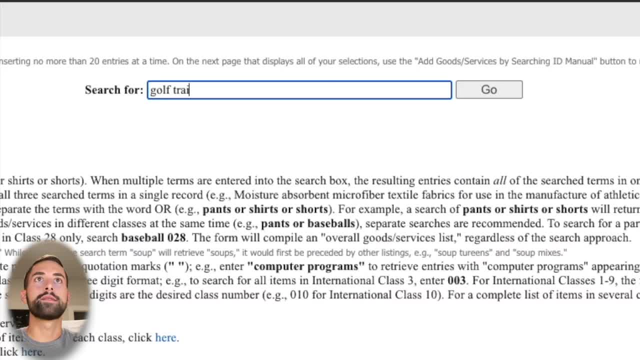 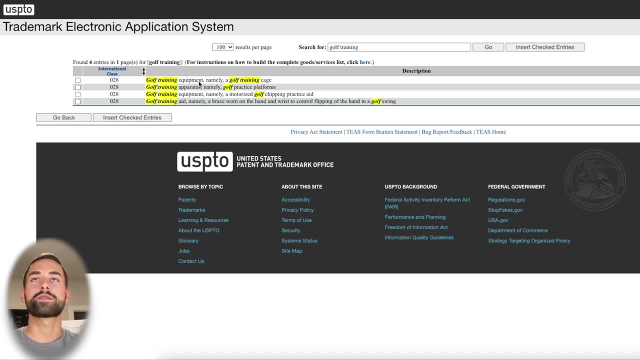 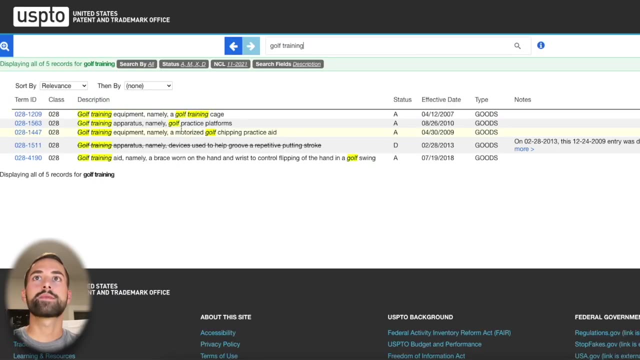 same thing, so i'm going to type in the same thing i typed before- golf training- and click go again. we found all the different descriptions and classes of good international classes here that relate to this golf training search term. as you remember before, if we jump back, this was the one that i want to trademark it under. it's a. 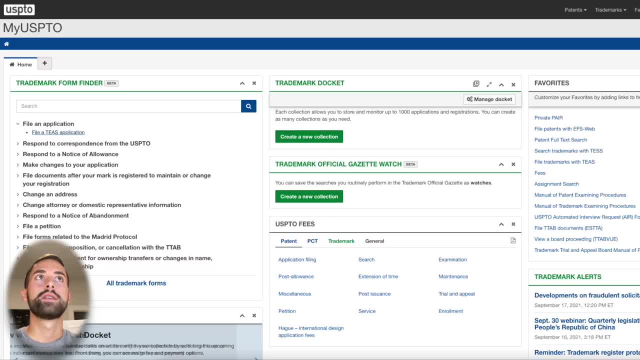 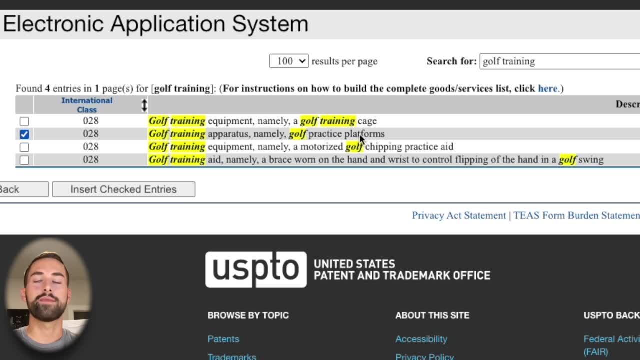 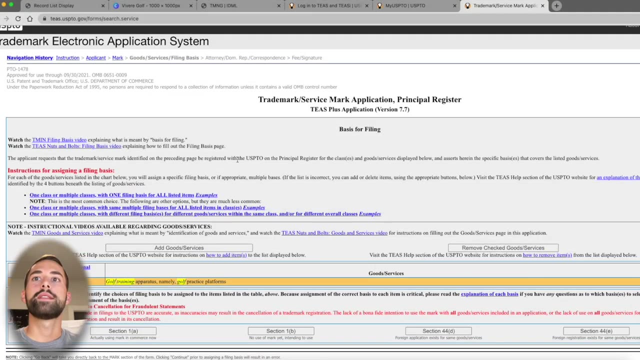 golf training apparatus- golf practice platforms. so we'll head back to the application here. then you'll select the class golf training apparatus, namely golf practice platforms. for this tutorial we are just going to be doing this single class, so we'll click insert checked entries and down at the bottom here you're going to see the classes that you are. 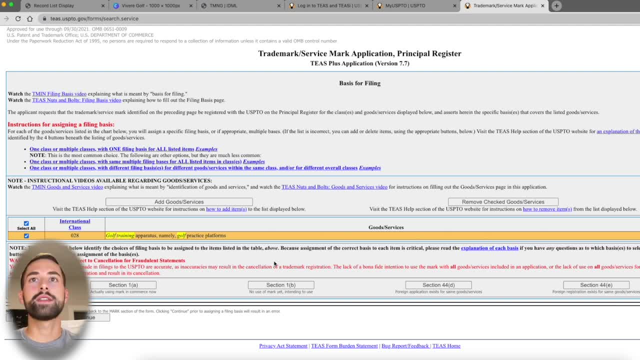 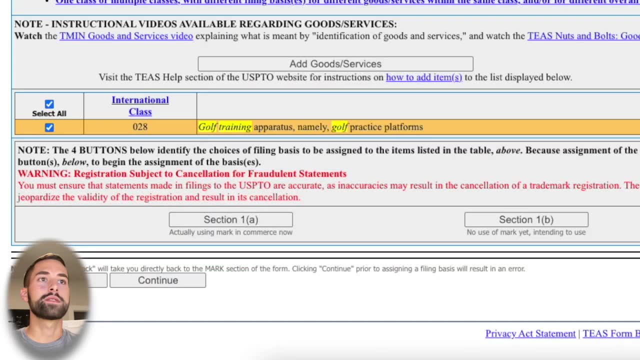 registering your trademark under. the last thing to do on this page is to assign a filing basis for this international class which is going to be shown down here. so you're going to claim: is it section 1a, 1b, 44d, 44e? and it's very convenient because i'm glad they put. 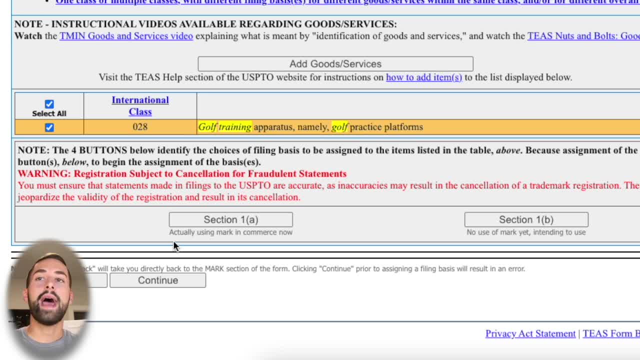 these under here so you can better understand what this actually means. so if you're actually using your mark in commerce currently, right now, which, believe it or not, you are allowed to do, if you just put the tm on it, you can do that. if it's not actively used, you're going to 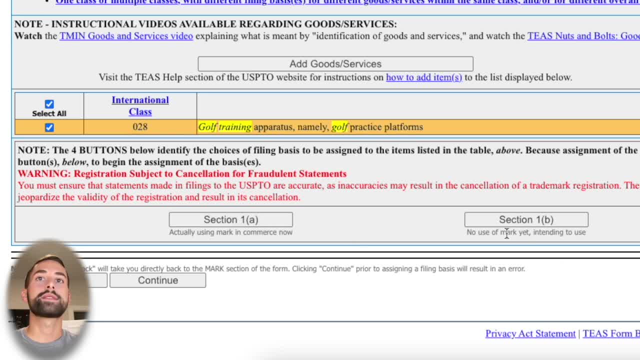 click 1a because you're using it in commerce right now for this brand. i'm not using it. i'm not selling any products under it right now. so i'm going to do 1b, which says no use of mark yet, but you're intending to use the other two here. they're for foreign applicants. it's very it's. 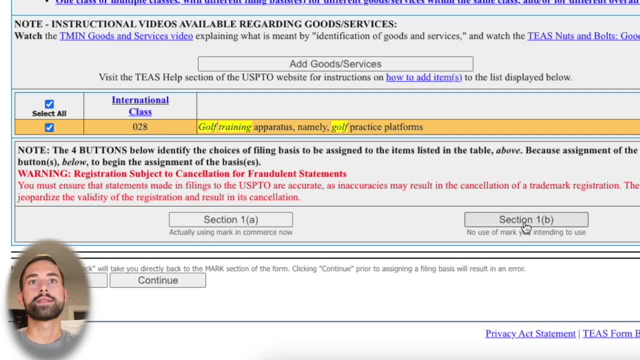 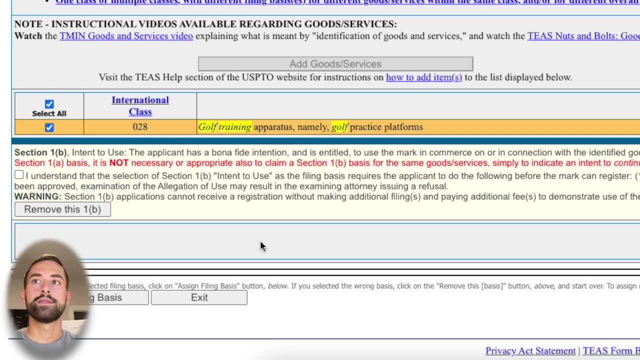 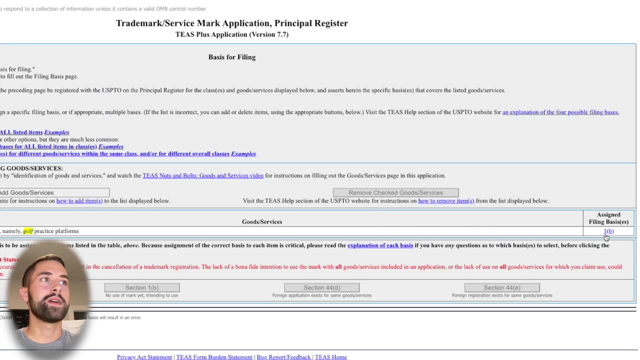 the same thing. it's actually 1a, 1b, but it's for foreign applicants, so for us we are not using the market in commerce, so we're going to do section 1b now. it's going to ask us to understand this. click i understand and click assign filing basis and at this point just verify that what you click. 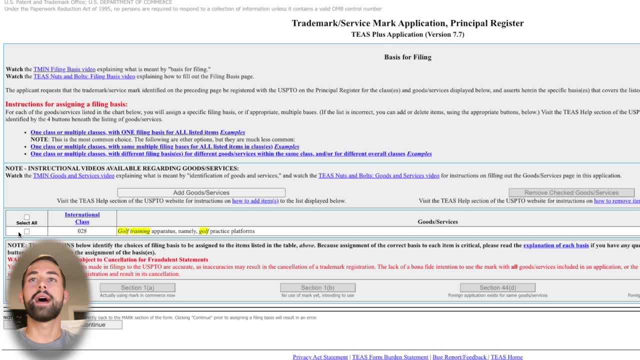 on's correct and then at this point just verify that yourlib is correctlyruled and not in this scenario. and also please make sure you forgot this at this point in your campaign from 1b before you drop in. so that's also important, but then you can also clean back up if you want. 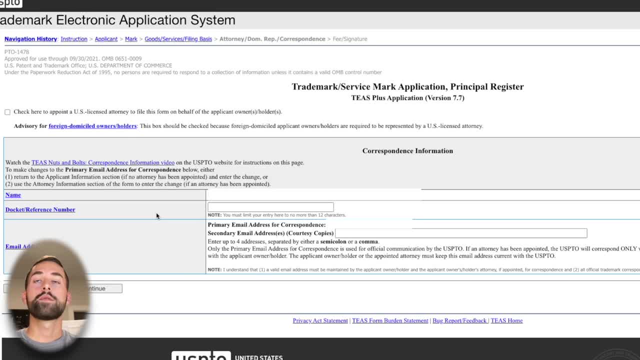 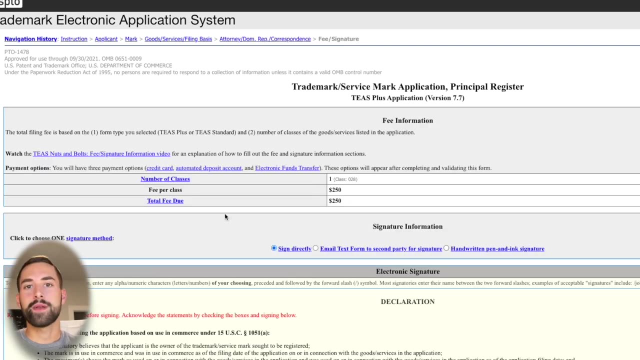 to walk our information out into our. Now is the part that we all hate, because you actually have to go ahead and you have to pay for this to be filed and then also sign off your name for this trademark brand. Again, it's going to be $250 per class if you do the Tees Plus and it's going to be $350 if you do the Tees Standard. 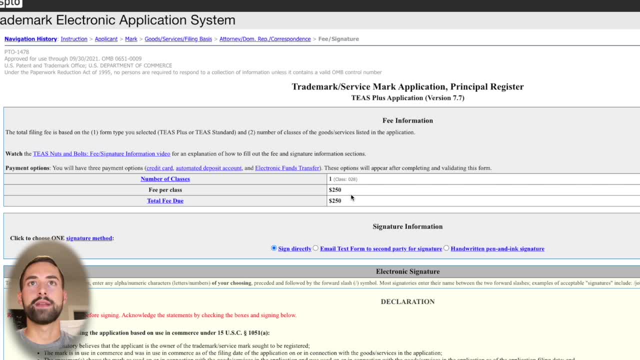 per class. Just something to keep in mind. You're going to have to pay some money, but if you do have a business, you can write this off your taxes as it is tax deductible. So confirm that that's correct and you don't have maybe two or three classes and you only wanted one. So we were only 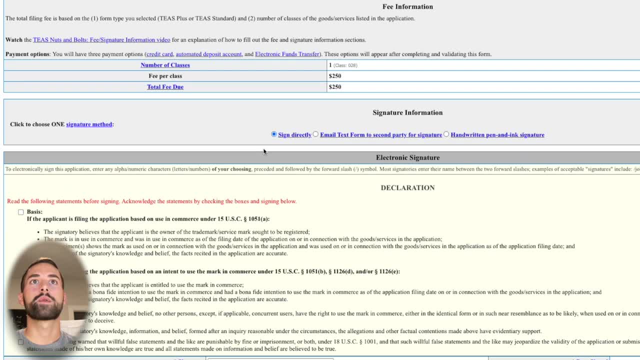 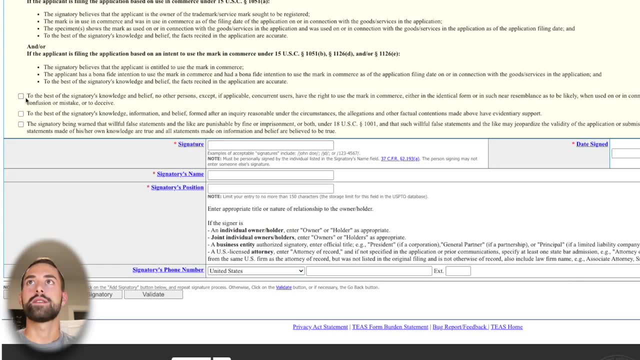 doing one. The amount is correct, $250 per- and then we're going to sign directly. You can hand write it and mail everything in, or you can just do it directly on here electronically. So you'll have to go through all this. You'll have to read the following statements. I've already done this. 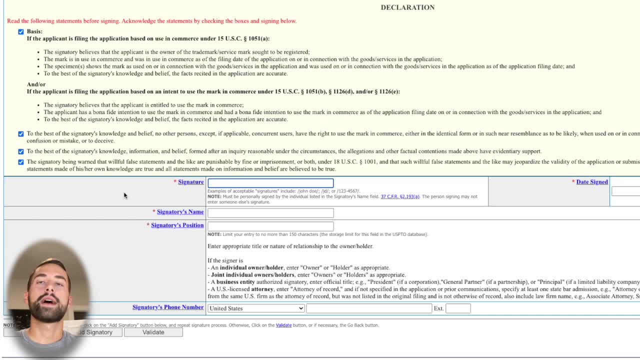 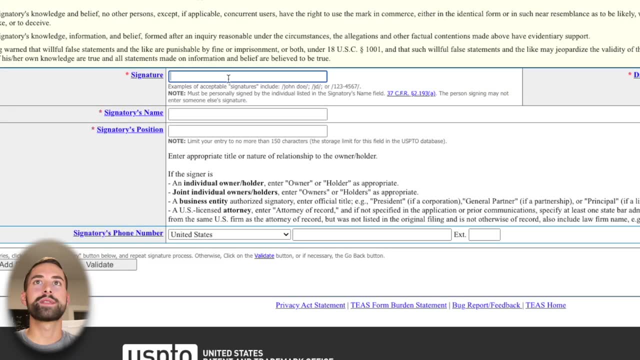 before and select all of them. Next we'll come down here to actually sign the application. Make sure you pay attention to this because it's very weird. whenever you do the signature, It's requiring you to put two forward slashes between your name in all lowercase, So put a. 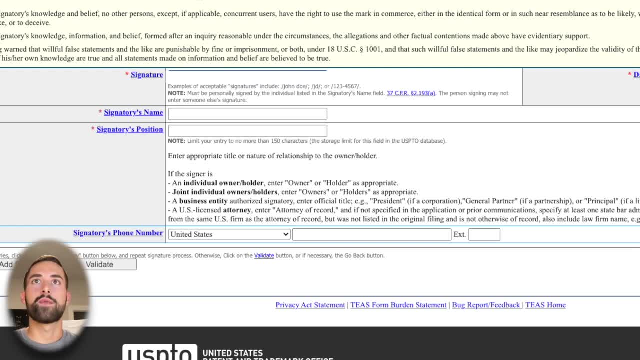 forward slash, Type in your name And then close it with another forward slash, I guess because it's alphanumeric. I honestly have no idea why you have to do that, but it's just something that they require For the names down here. you do not have to do that. You can just type in your name as is And then for the position. 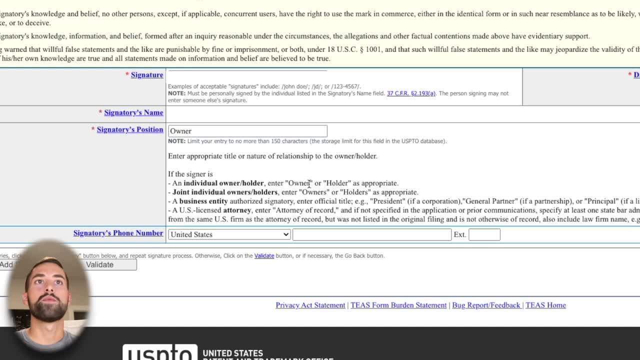 I am the owner of my company, So I'll put owner in. If you have a formal role for your company that you work in, make sure you put that there. or you can just type in individual For date sign, just click it, It'll auto-populate Make sure that's the correct date And then go down to 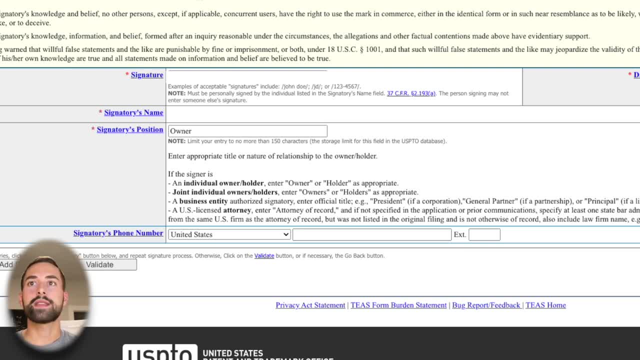 the bottom here. If you have more than one owner that needs to sign, click the add right here. You can add them, just like we did to add owner before. If not, if it's just yourself, like we're doing here, click. 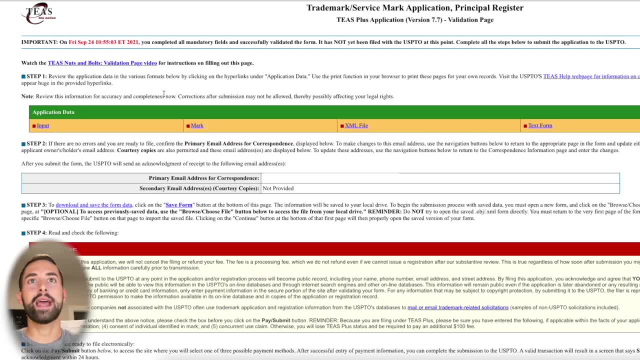 validate Okay, And once we've done that, we are basically completed with the application. We've completed all the mandatory fields. The USPTO website is just going to ask us to go ahead and to review everything to make sure that's correct. Do not be lazy. Make sure that you review. 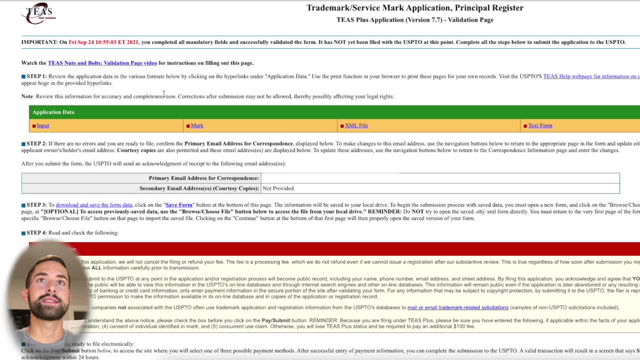 everything, because this is your one shot of branding this and you don't want to waste any money, Trust me. So go down through all these steps, go through all the data just to confirm that your name's right, the trademarks looks correct, the logo's correct, the descriptions there, all of the above. 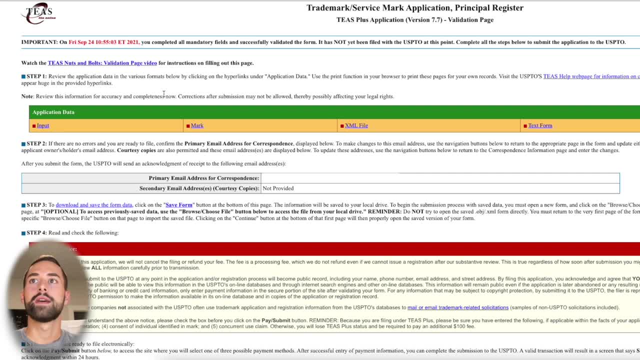 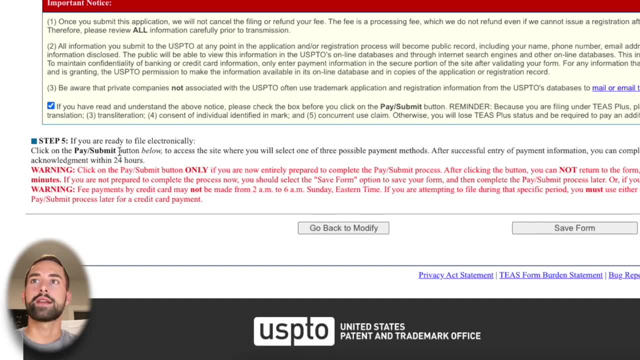 check everything And then, once you do, you can go ahead and you can go through all these checks. You can check this right here. It just goes over the payment information and go down to step five where it says, if you're ready to file electronically, click on pay and submit. 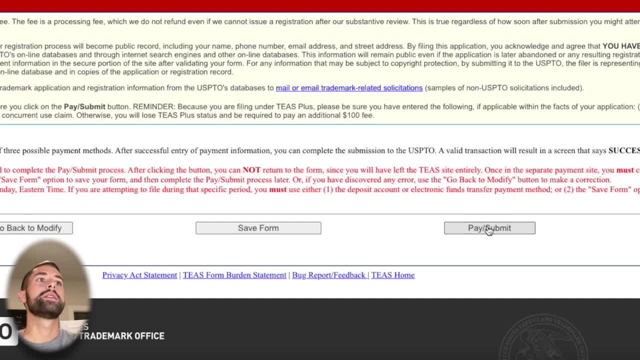 So this is the final step. Once you click pay and submit, you'll be brought to the screen where you'll input your credit card And then you'll be able to go ahead and go ahead and submit your credit card information or whatever you're using to actually purchase this filing. 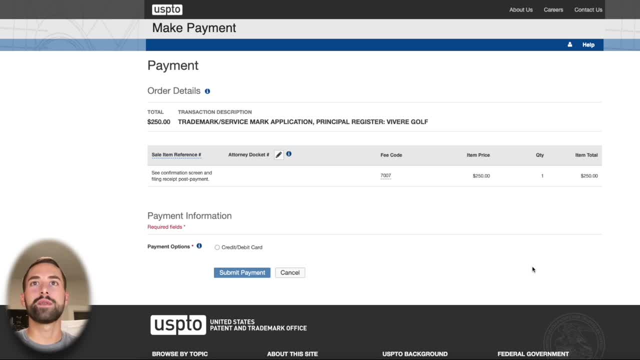 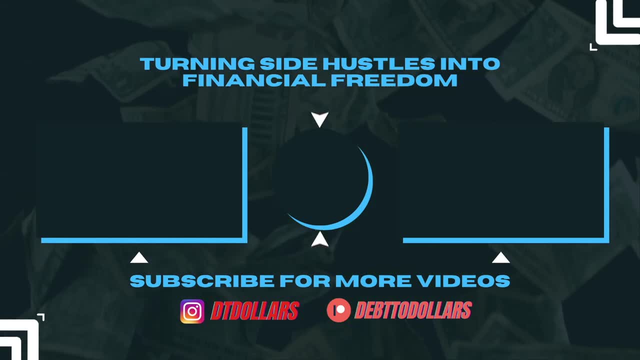 All right guys. thank you for watching. I hope this gives you more insight on what to do when filing your trademark application. It can seem very daunting, especially with all the little nuances like the signature there at the end, but you do not need an attorney. 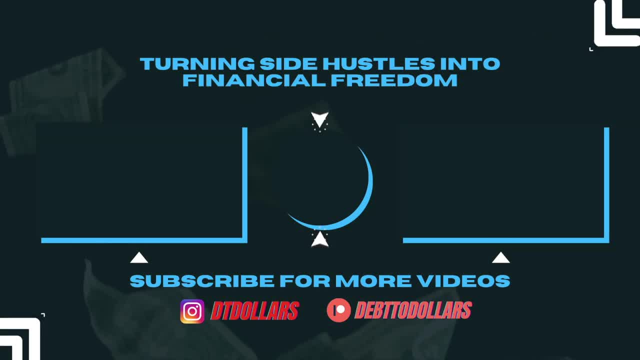 If you do want to go ahead and get an attorney, I do recommend doing the Amazon IP Accelerator program. It's a little more expensive, but that way you make sure you get it done correctly the first time.